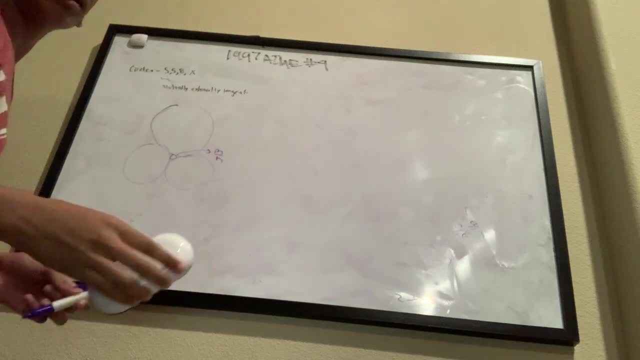 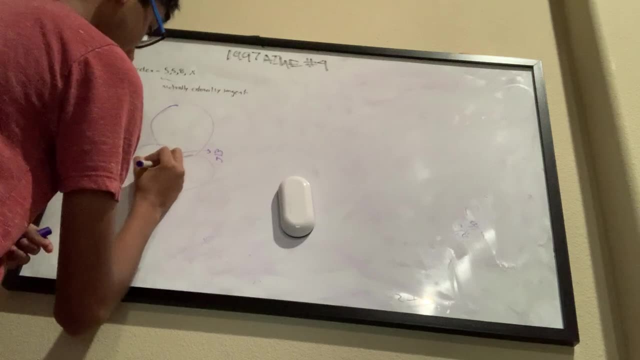 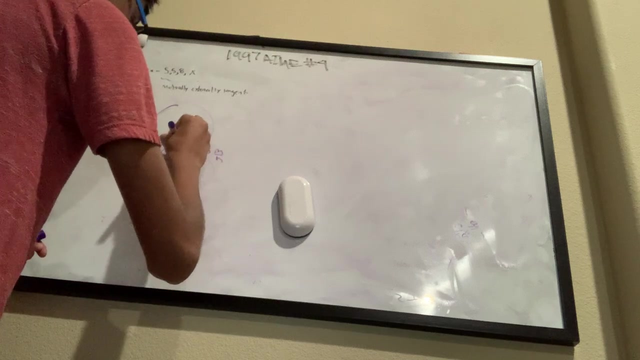 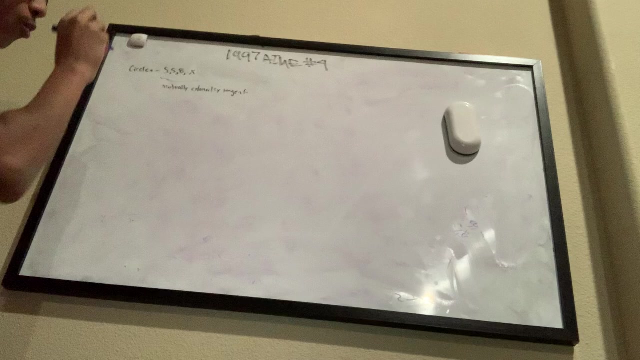 really we do not need this. We could do it in like a triangle way, Like kind of like. we could probably like try something like this connecting the centers of any one of all of them, Something like that. But honestly, I think using the theorem is way easier. So, because they're mutually so what is the Descartes circle formula? Well, I'm going to use 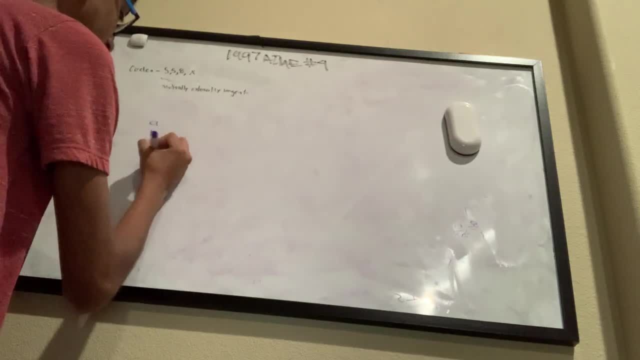 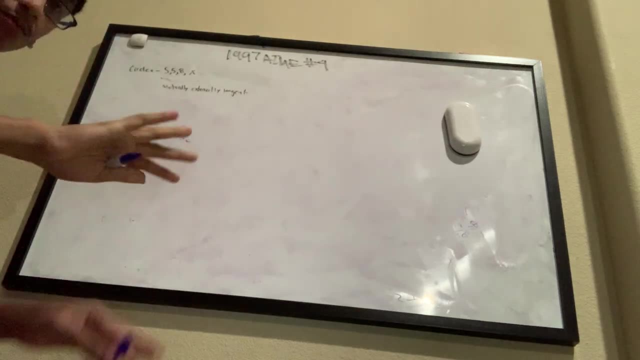 notation a, b, c and d. so these are going to be the radius, and you may have not learned curvature, but i'm just going to say now that's going to be needed. just pretend what, don't care what it is now: a, c, b, c, c, c and d, c. yeah, c, c may be a little bit confusing, but basically the theorem states: 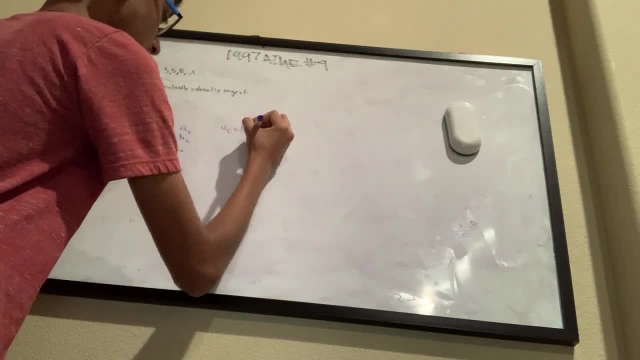 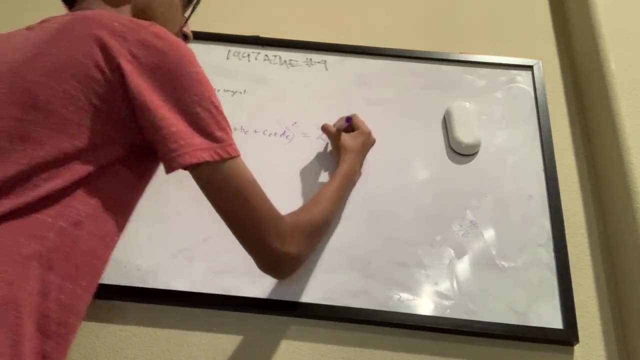 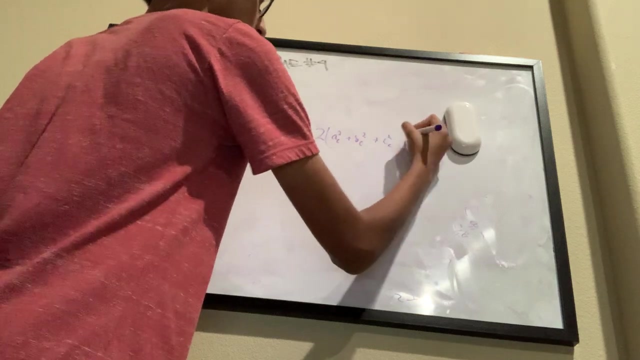 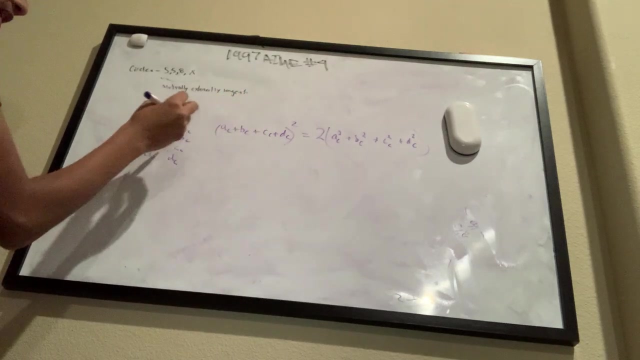 that a c plus b c plus c c plus d c squared is equal to two times a c squared plus b c squared plus c c squared plus d c squared. now we need to find d c. okay, so we let's. so how, what we're going to do and, by the way, we're going to simplify this a. 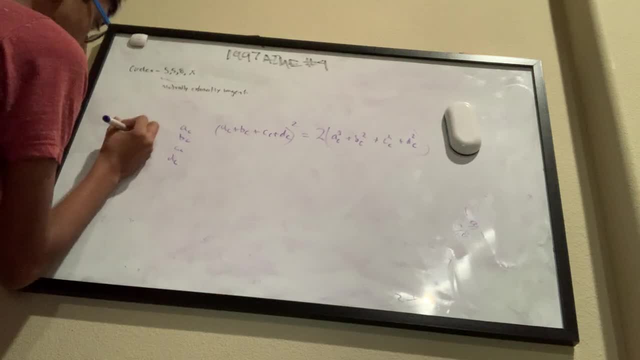 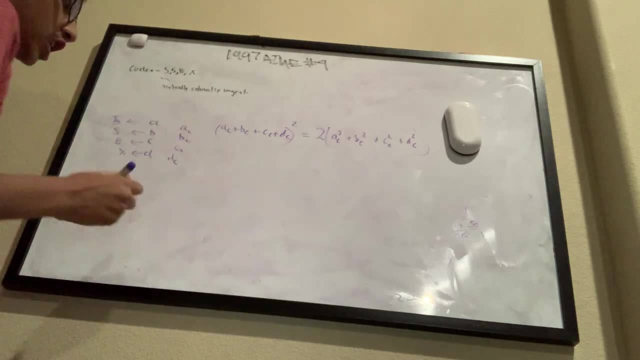 you. it's going to a is just going to be radius. so we're going to say five here, five here, eight here, and then let's going to say x here. now the curvature is basically just plus or minus one over r. this is important: plus or minus one. 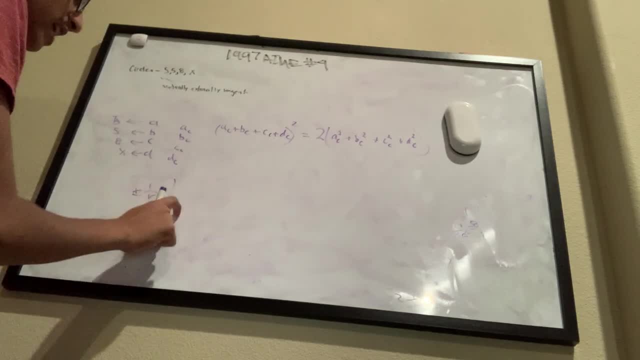 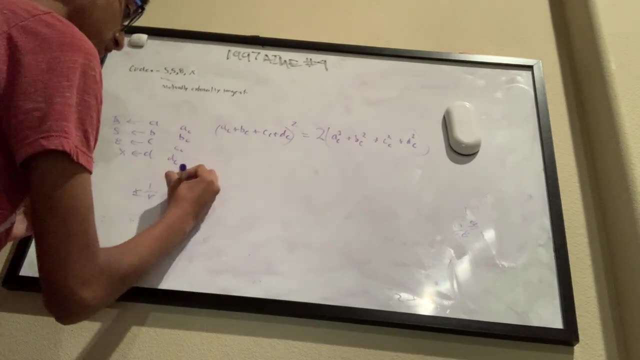 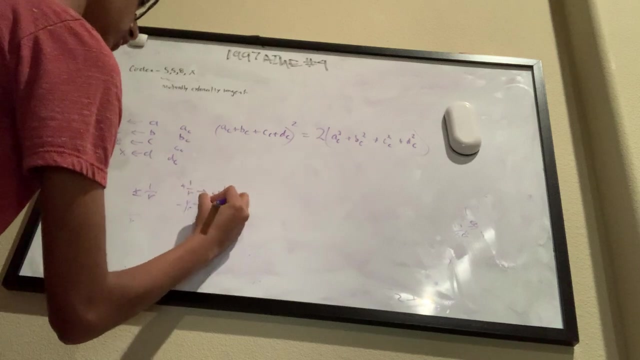 over r, and that's known as the curvature. now how do you know if it's plus or minus? well, if they are x, if this circle is externally tangent, it's positive one over r. so that's, if it's externally tangent, it's negative one over r. if it's internally tangent, 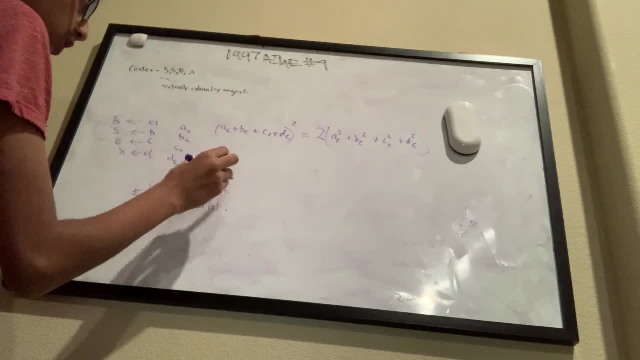 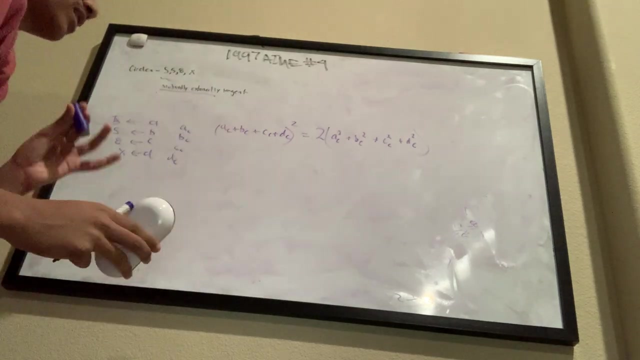 now, what is such important is seeing this problem. it says mutually. externally, this means that all of them are um, are, uh, are, uh, um. all of them are a positive curvature, which is good, because definitely you use it for a problem, so we can, obviously. so what is our curvature? as well, we. 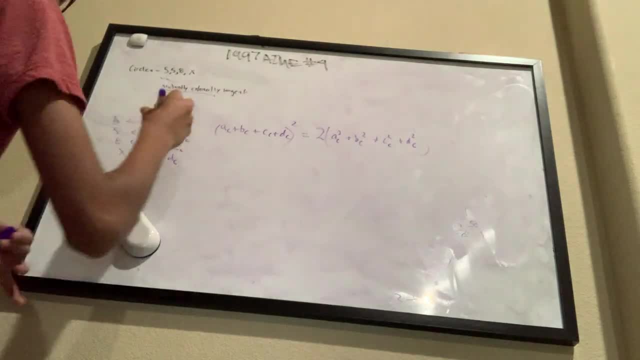 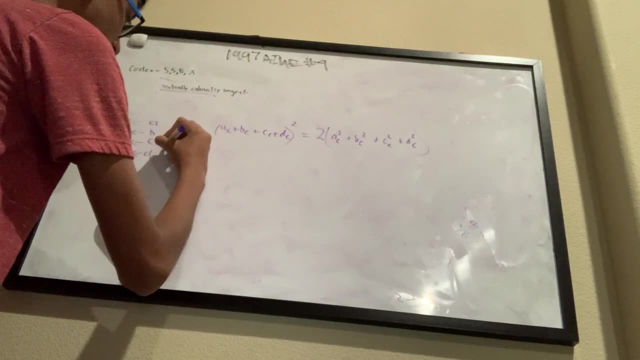 say it's plus or minus, one over r, and that's if it's externally tangent. it's negative: one over r, minus one over r, and we know now it's one over plus, one over r for all of them. so ac is equal to one-fifth, this is equal to one-fifth, this is equal to one-eighth and this is equal to one over x. 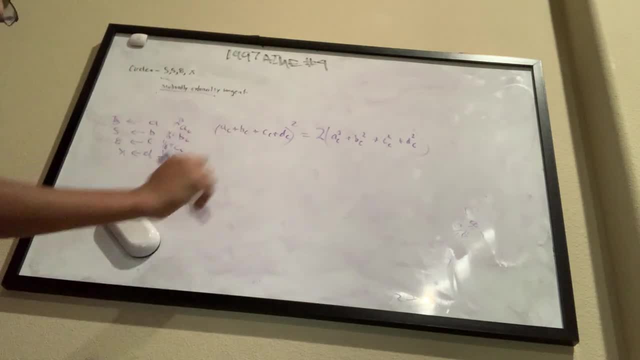 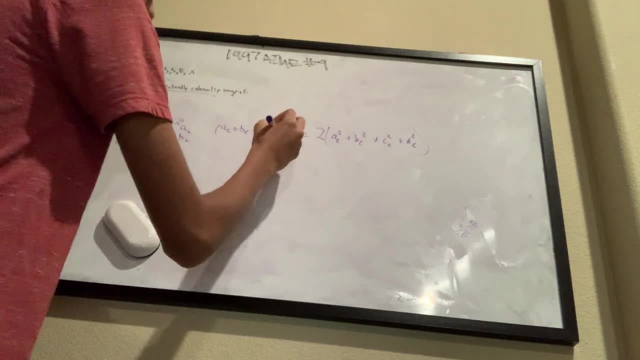 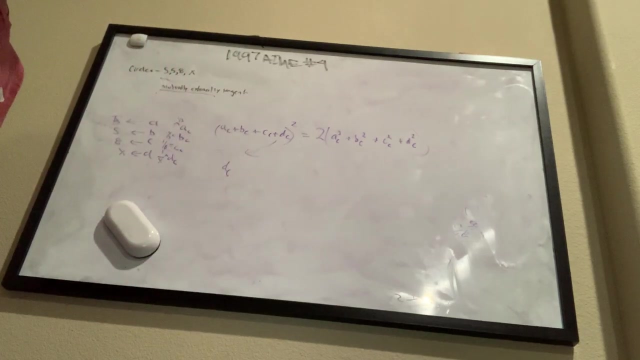 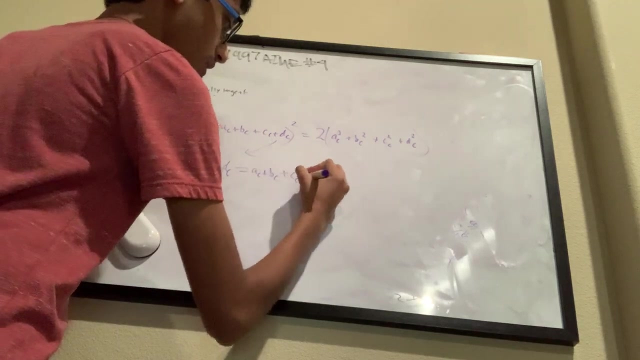 but before we can plug this in here, yes, but let's try an easier way. now i'm just going to say it off, but this could be pretty easy. there's a way to just get dc by itself and that way, that way. that way is basically it's just: dc is equal to ac plus bc plus cc plus the square root. 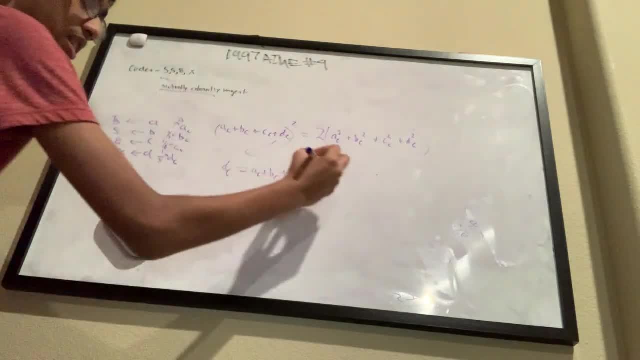 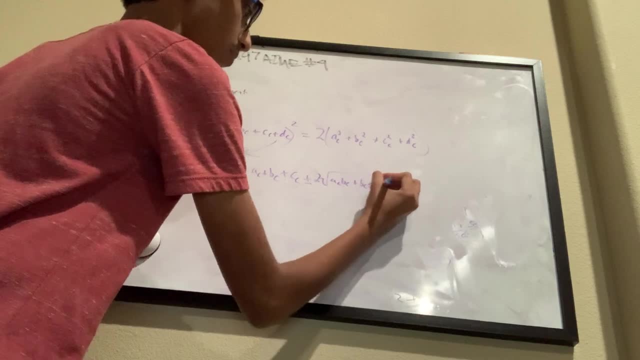 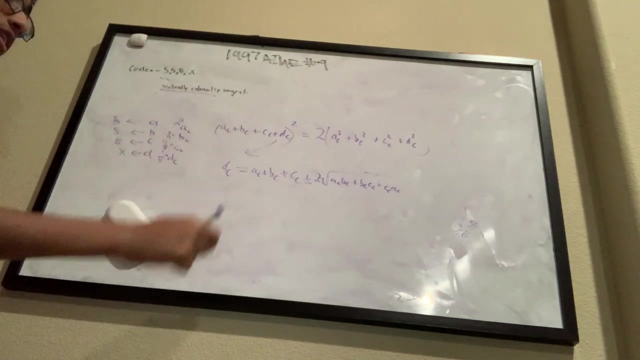 uh, plus or minus, basically. uh, i think uh, two times ac, bc plus bccc plus ccac. so that is how we can get dc. and yeah, this could be easy, but it's just a way to get dc by itself, and that way it's just a way to get dc by itself. 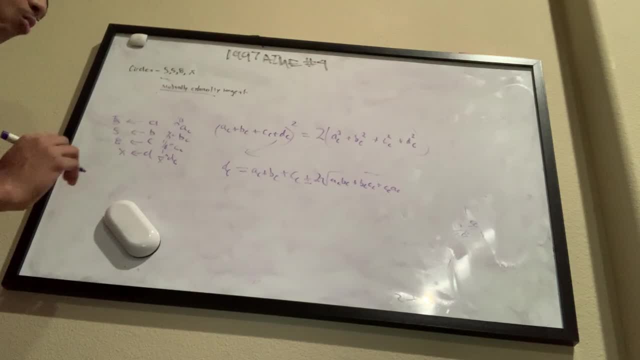 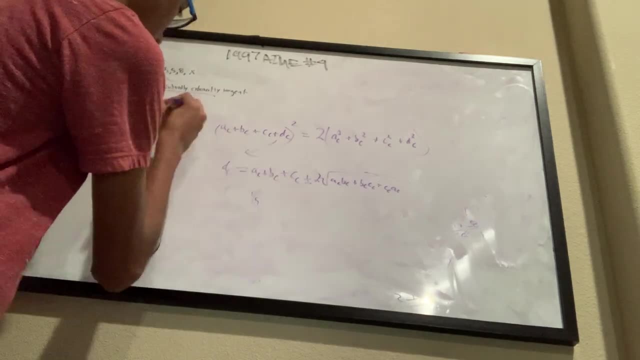 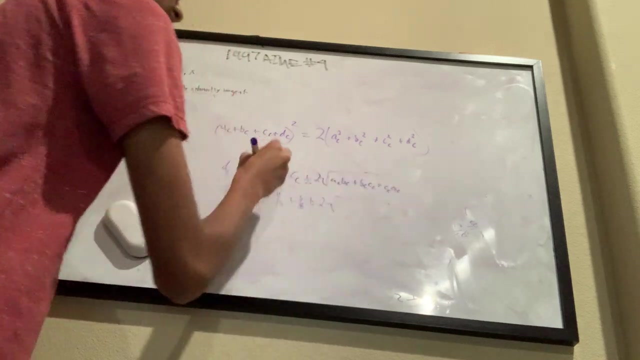 easily, uh, just factor out in general. so what is it going to be? well, let's think about the ac. we said is one-fifth right there, plus one-fifth plus one-eighth, plus or minus two times the square. ac times bc is one over 25. uh, bc times cc is one over 40. 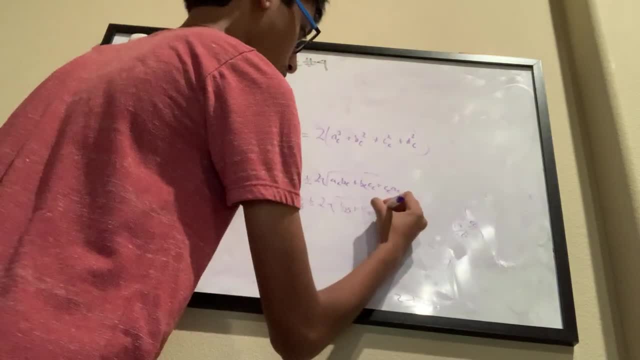 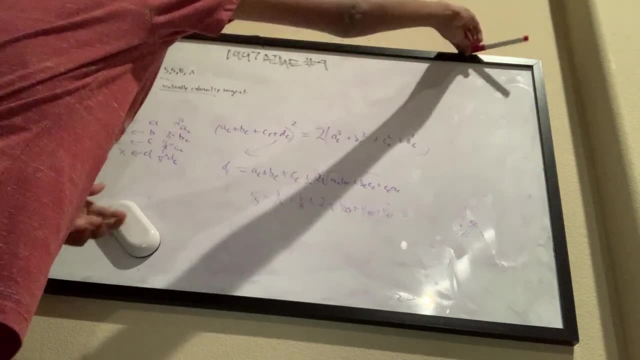 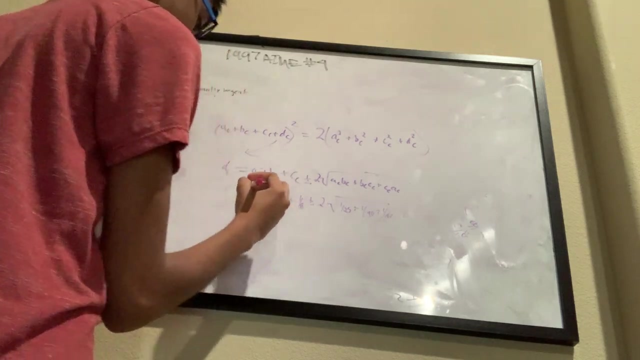 and then cc, uh, cc times. ac is one over 40.. this one's running out, so let's just solve this. so this becomes two-fifths plus one-eighth, which is just um. two-fifths plus one-eighth is just uh, if i'm not wrong, 21 over 40. 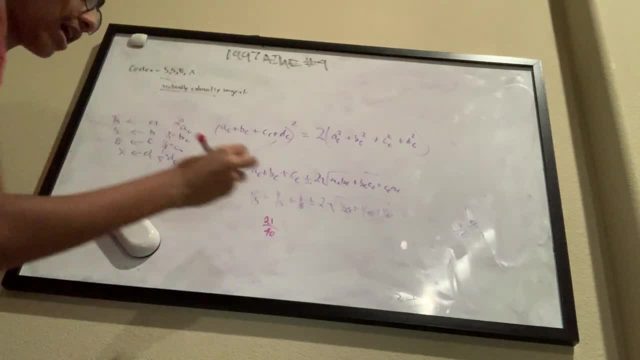 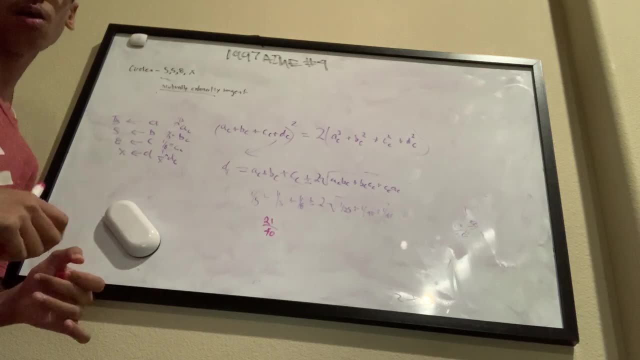 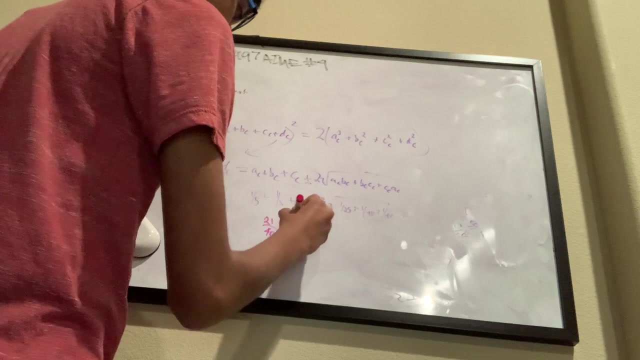 and that's going to be a plus or minus. um, well, the thing is it's plus or minus, but we know, uh, we want the, we want the large, because it's a plus or minus. so we're going to externally change it. it's just going to be plus. so it's going to be plus two times the square. 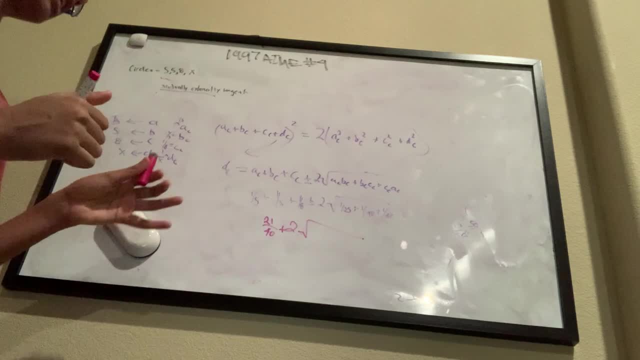 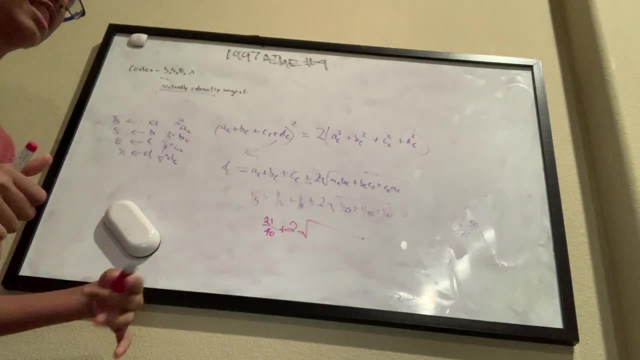 root and of course, you can always assume it's going to be plus and i'm pretty sure, if i'm not, yeah, if i'm not wrong, if you do minus, you're going to get a negative, and you, if it's a negative curvature, um, i mean, you could solve it, i mean, but you know you want to you. it's best to assume.